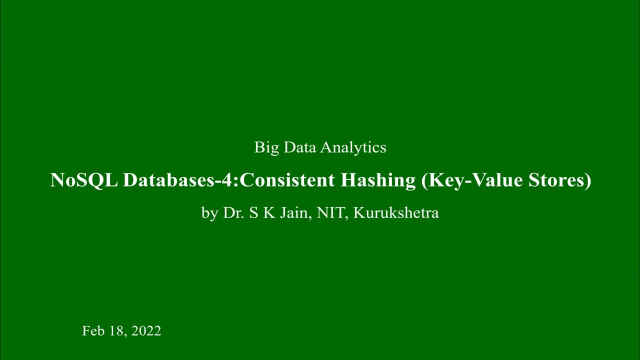 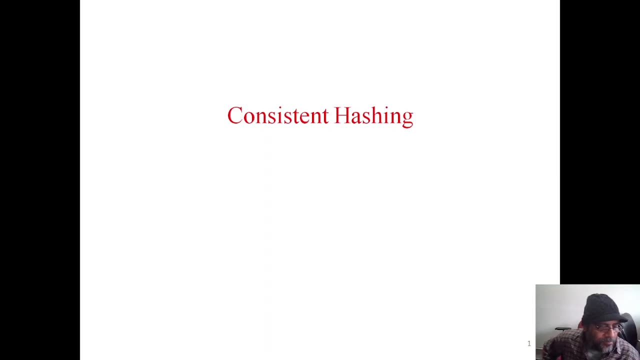 So in previous class we were discussing key value data store. that is simplest form of the NoSQL database and we discussed there are only three operations which are supported by this key value data store: to keep data in the data store, to retrieve and to delete. 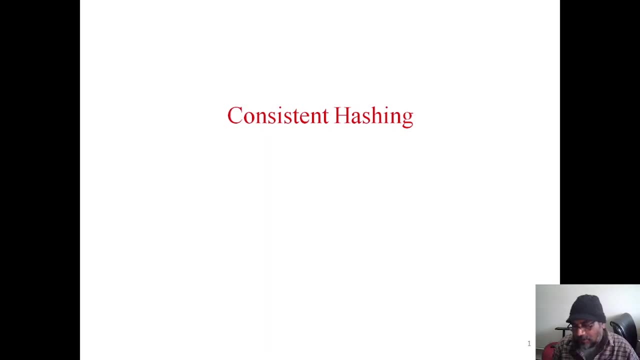 There is one important factor that is called consistent hashing and we have, suppose, very large number of key value data And we have to store them on several different nodes or several different storage devices, And we want that our data should be stored uniformly or in some balanced way so that 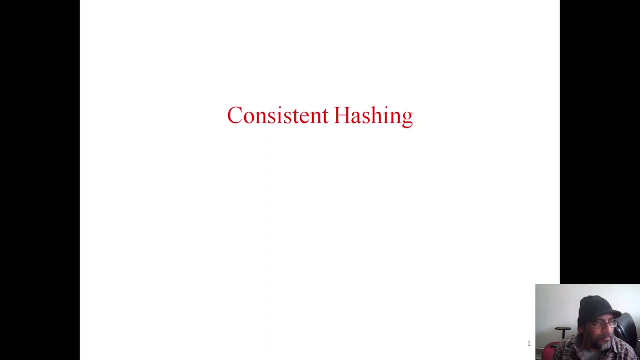 each node have equal amount or equal storage devices. So we are going to discuss how to store data in capacity and how it can be done automated. So one solution is this consistent hashing that we will discuss And second, we will discuss how relational data can be converted into key value data. 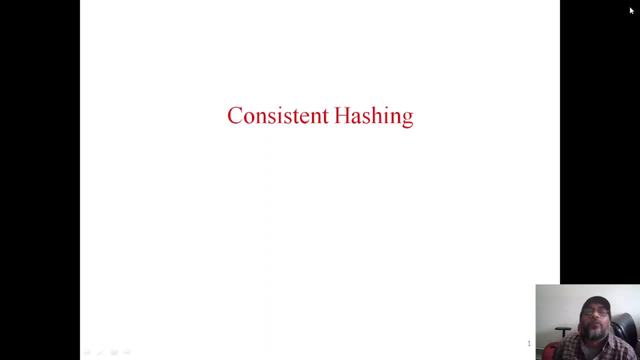 Two things we will discuss today. So hashing- Hashing- you know already hash function. We have some value and when we apply hash function we get small size value set or we get values only a limited range. So with the help of hash function for very large number of values, 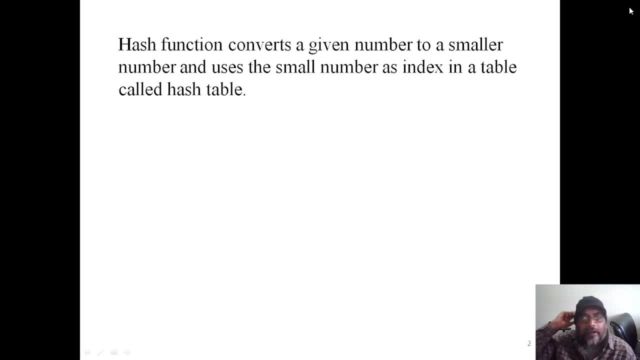 We can make one hash function. So we can make one hash function. We take one index small table and for this purpose we make a function that we call hash function. So hash function converts are: given number of smaller number. hash function converts are: 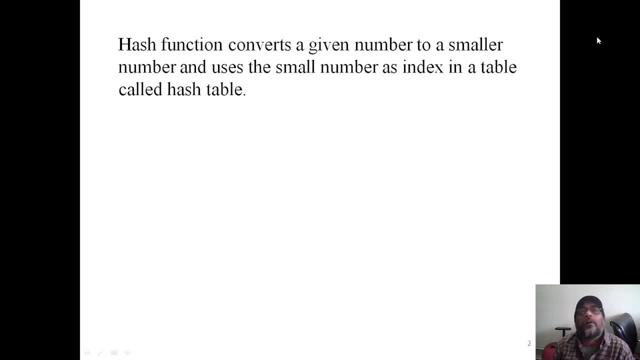 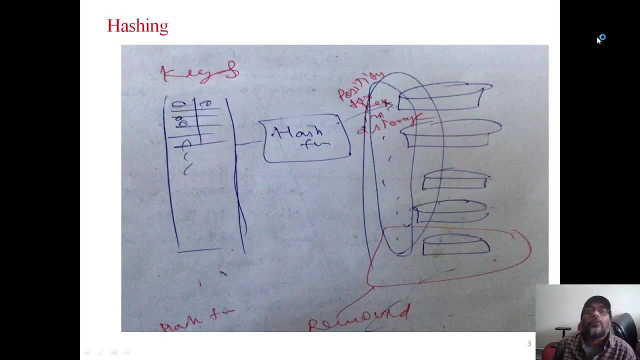 given number to a smaller number and uses small number as index in a table called hash table. Ok, So in practice, suppose this is the key value data and if we apply hash function and we make that hash values, they are one, two, three, like, and suppose I have five data stores for. 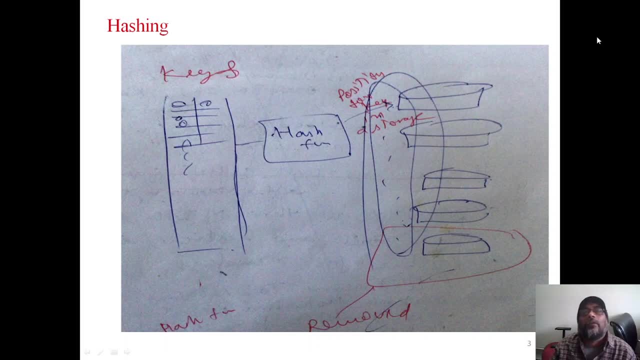 five nodes And based on values generated by hash function: one, two, three, four, five, the values key. based on the key value, the hash values are generated and the data values can be stored in this form. but suppose what will happen if one node is removed from this cluster? 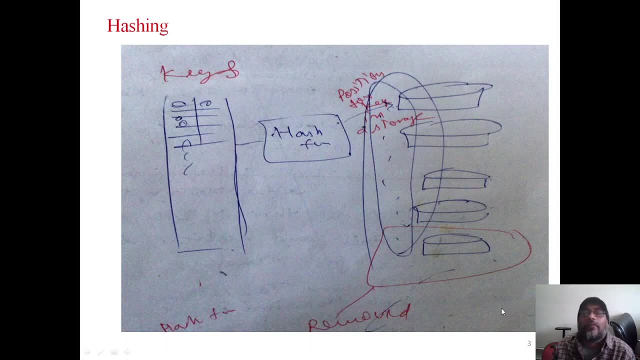 the problem may be that we have to reassign all the data values because now hash function is changed, or the values that were earlier being generated by hash function. now it has lesser number for hash function that was earlier generated. so how this problem can be resolved? so that technique is simple technique and it is called consistent hashing. 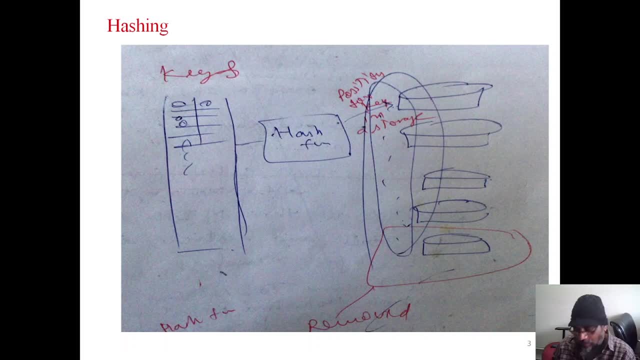 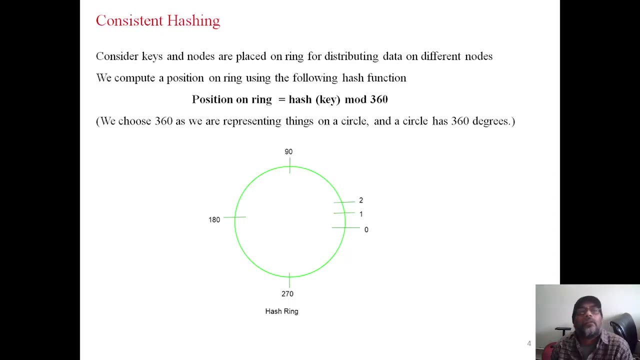 so, before coming to the actual explanation of this consistent hashing, we have one small experiment that will help us to understand this consistent hashing. so suppose keys and nodes are placed on a ring for distributing data on different nodes. so this is the ring, and here we compute position of ring. 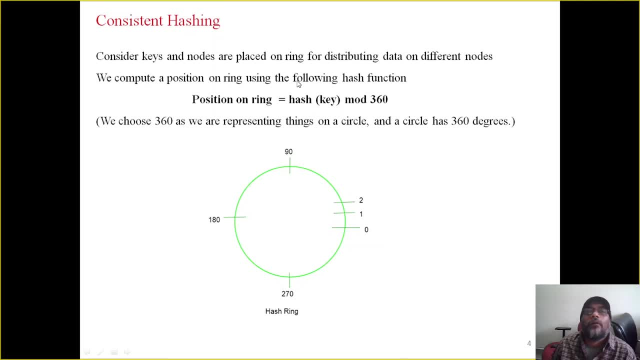 position on ring using the following hash function: so on this ring we have, because it is circle shape, so we can also imagine in form of 360 degree from center. so if any position on this circumference, on this ring we have to identify, one argument can be in terms of angle. 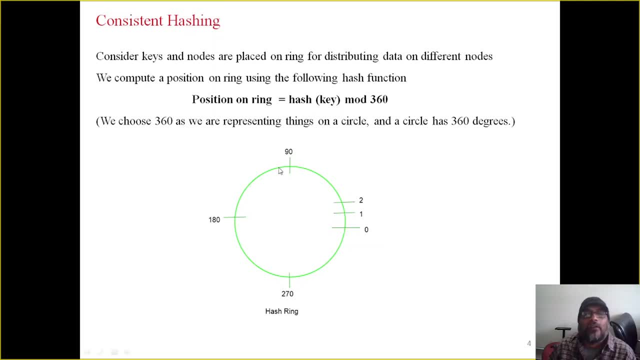 so 0 degree, 1 degree, 2 degree, 90,, 180,, 270 like that. so they can also be used for referring the position on this ring. so this is the to identify to make any position on ring. this function is used as E mod by 360. 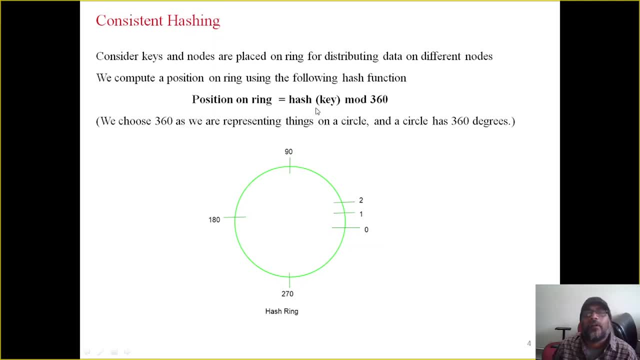 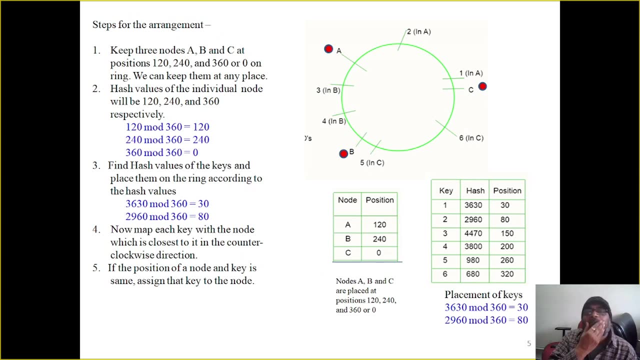 so we choose 360 for representing the things on circle as 360 degree. so now what we shall do? we keep node on the ring and then we will apply hash function on the data key and it will generate the value, hash value- and that value may be kept on one of the nodes. 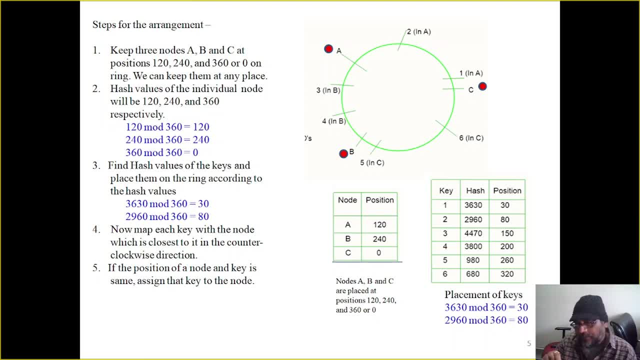 and on this node we have to keep that data value. we will make some rule. so you see here, suppose there are 3 nodes, keep 3 nodes, ABC, at position 120, 240, 360 or 0 degree, this red color they are representing. 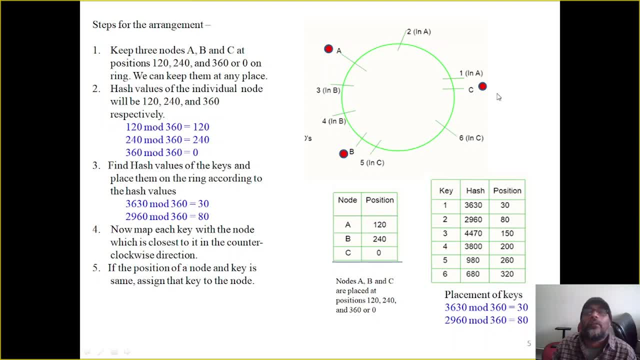 A is 120,, 240 and 360 on ring. we can keep them at any place. just for convenience I have taken 120 and 240, but you can keep anywhere. ok, later on we will come to know so hash values of individual node here will be. 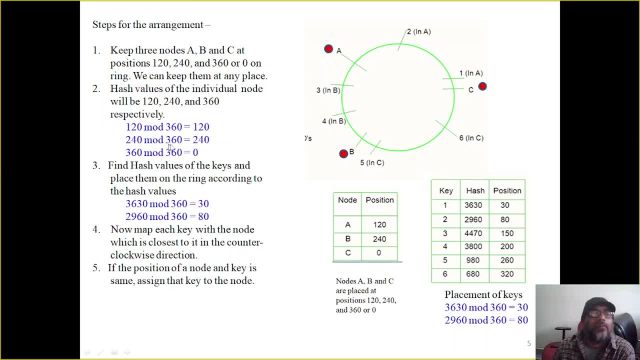 like 120 mod, 360, 240 mod. so these values will be. so they are the positions on this ring. find hash values of keys and place them on the ring according to the hash values. so this is node A, node B, node C and they are the key. 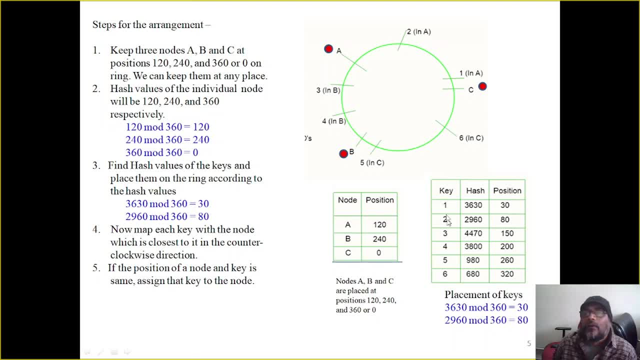 of my data values. ok, so these key, basically 1,, 2, 3, I have written for convenience, so we are considering they are the actual value that will be hashed. so after hashing we get some value here and that value is corresponding to position on ring also. 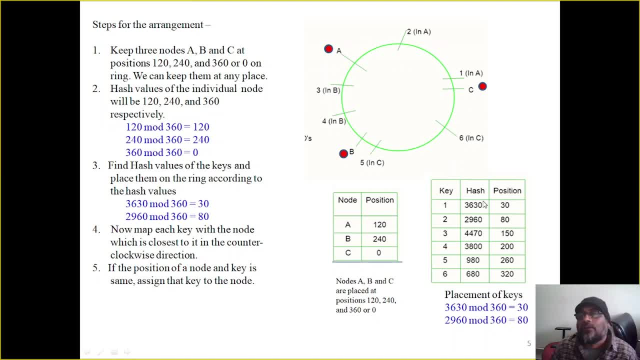 because we have taken 360 mod, so this mod 360, 30. similarly, when we divide by 360 modular arithmetic, so we will get all these values. ok, so 3093 mod 360, it will come out 30, so 30 will be placed here. 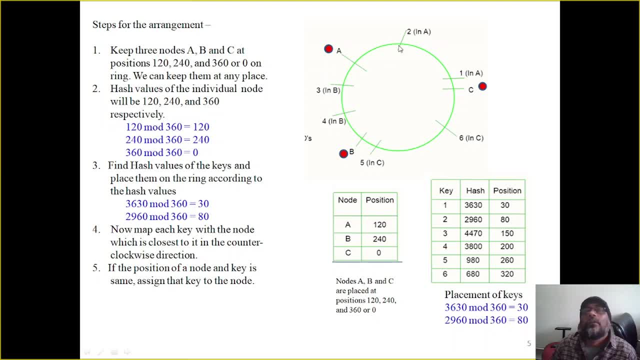 ok, so this is written 1, second 2960 at 80 degree. so this is 2, this is key 3, 150, then 200, 263, key 4, key 5 and 6 keys. they have been kept here. now we make rule that. 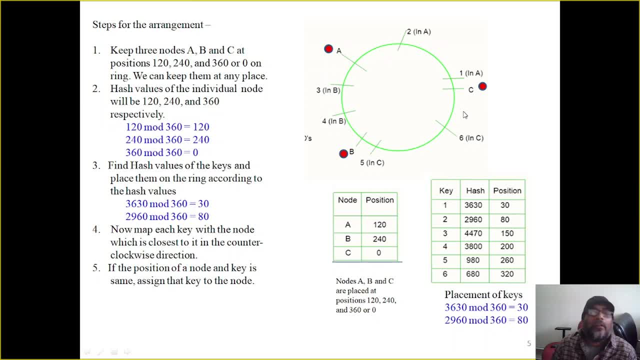 when we move on circle in anticlockwise and whatever node comes we assign these key to that node. ok, now map each key with the node which is closest to the closest to it in counterclockwise. so suppose 6 key now we will keep or we will store. 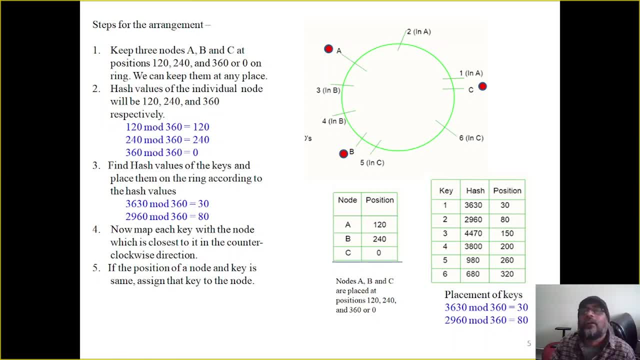 these key on which node? so I make that we move in counterclockwise and whenever new first node appears to it it will be stored. so you see, when we move counterclockwise from here, key 1, key 2 will be mapped to A. 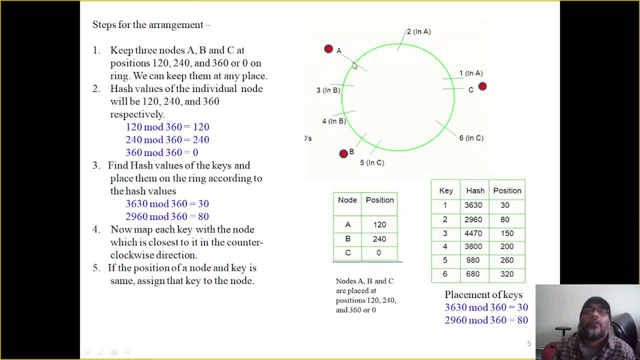 after 1 and 2 we come A, then key 3, key 4, then we have here. so key 4, key 3 and key 4 will be mapped to B. it is written here in B in B. it is in A in A. 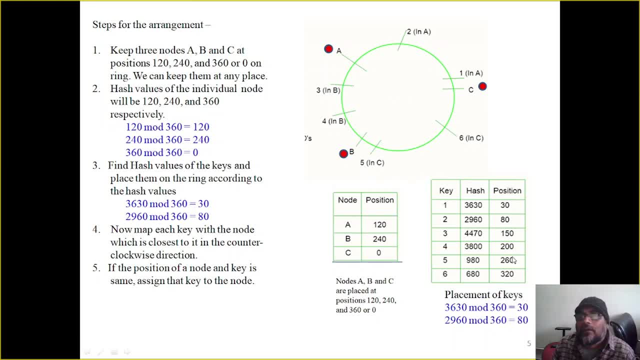 and this 5th and 6th key at angle to 6320. they will be mapped to C. ok, it is also written in bracket. ok, so 6 key here. they are really very large number of key in practice. so they have been mapped to. 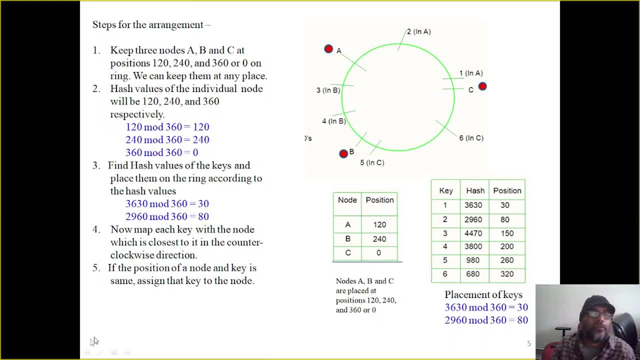 these node A, B, C. according to this rule, now map each key with the node which is closest to it in count and counter or anti-clockwise direction here. this instead of anti-clockwise clockwise rule can also be made ok, so there is no need. 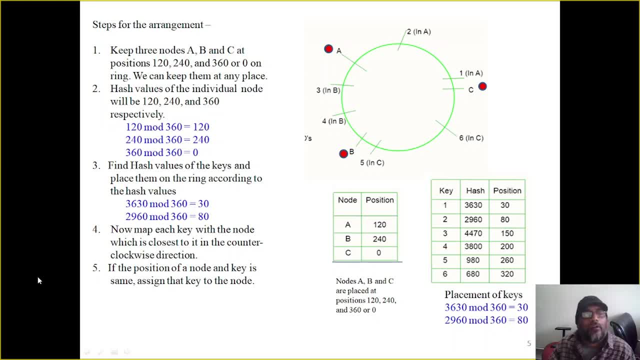 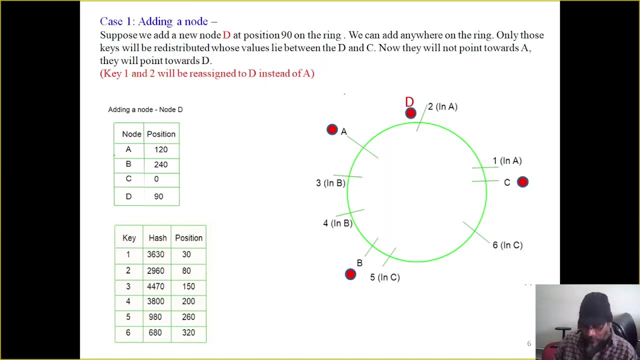 it is not necessary always. you go for counterclockwise. if the position of the node and key is same, then assign the key to the node. this is rule. so this is the experimental setup. now we add: we add a node in cluster. ok, you can also assume this is a cluster. 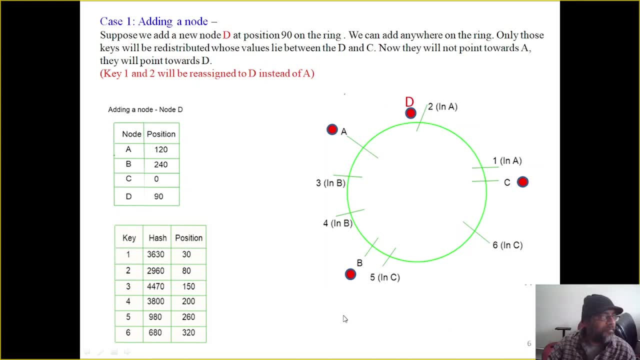 so we add a new node in cluster and we check whether the key that was earlier assigned have disturbed and how they cannot be made so that reassignment should be minimal. so case 1: add a node. suppose we have, suppose we add a node, a new node D. 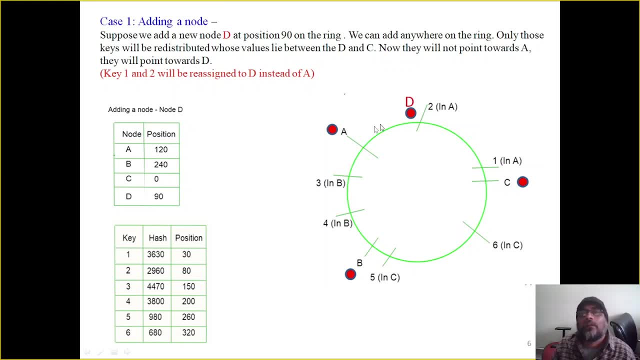 ok, so you see here, this is new node D at 90 degree. it is shown here red color D. so suppose we add a node, a new node D, at position 90 on the ring. you can add anywhere. ok, so we can add anywhere on the ring. 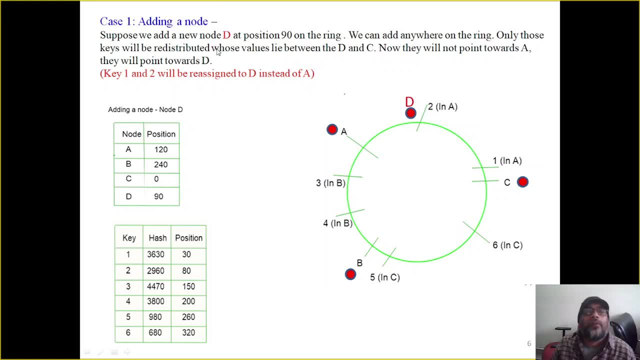 only those keys will be redistributed whose values lie between D and C. D and C now they will not point to A, they will point to toward D. you see, here, when we add this new node- and earlier our rule was- the keys will be assigned to that node. 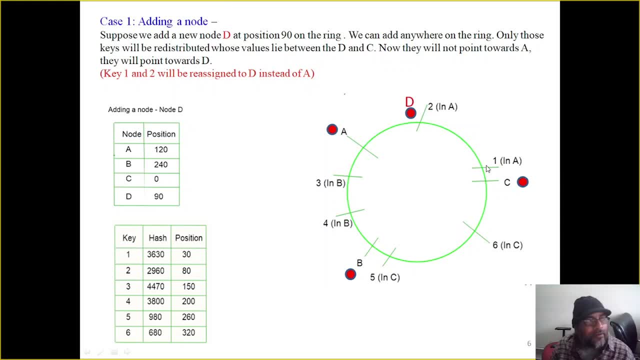 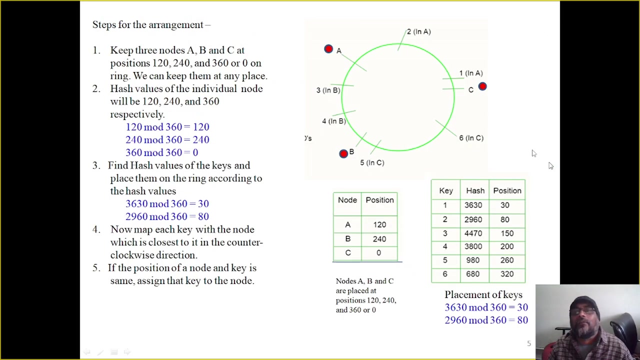 which are close to the close to it when we move anti, counter, anti clockwise or counter clockwise. so you see, here D is added. so you see the first key and second key. now they will be assigned to D. earlier, first and second were being assigned to A in this experiment. 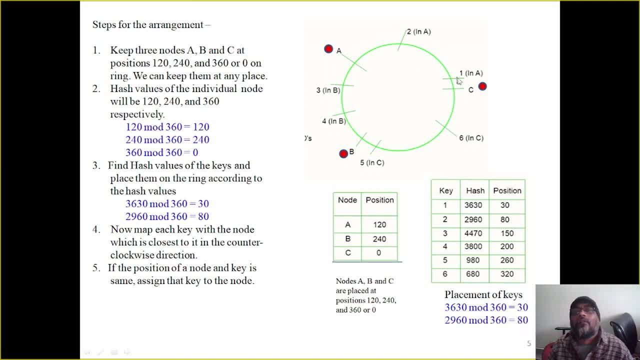 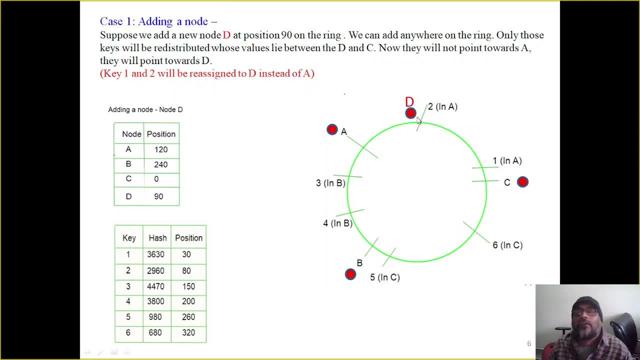 1 and 2. A now 1 and 2. they are close to D, so they will be reassigned to D. so only these two keys are disturbed here. rest key will remain as such. ok, 1 and 2 will be reassigned to D. 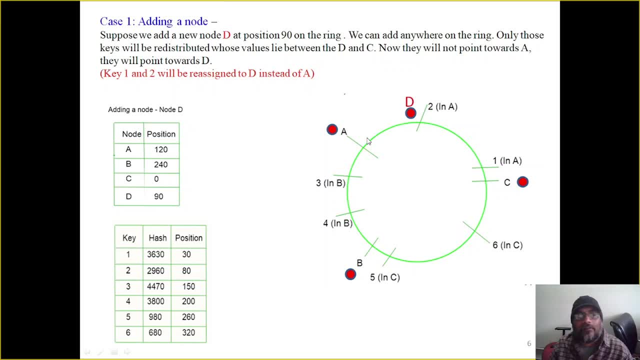 instead of A, instead of A now. so this change we have to make here and here you see the new position. what happens here? node A, node B, node C, node D: they are the angle and position shown here, key values. ok, so now this first and second will be assigned to. 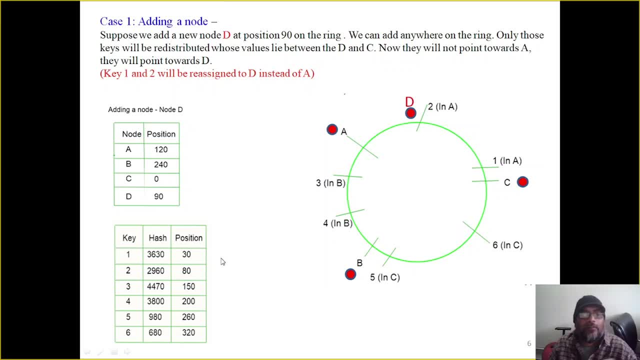 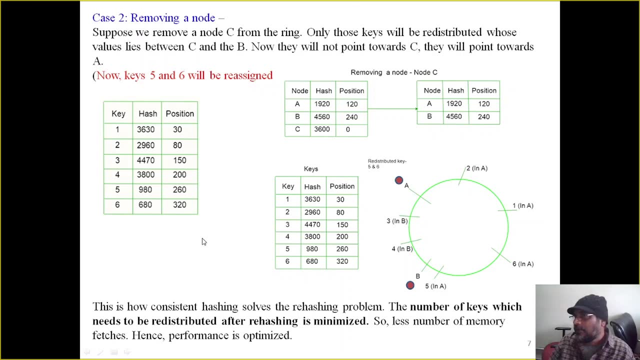 D. ok, I have not written, but I should write it here, ok? second, if we remove a node, then what will happen? suppose we remove a node C from the ring earlier. here we have this C node and now we are going to remove it. so this is the picture. 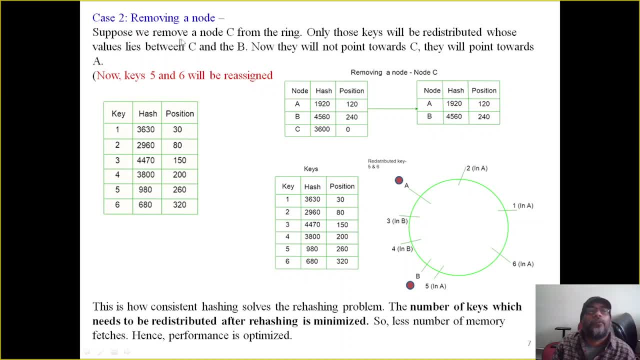 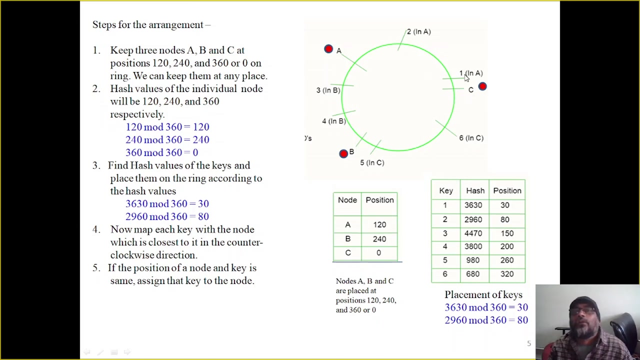 and A and B are still present. suppose we remove a node C from the ring, only those keys will be redistributed whose values lie between C and B. now you see, when we have removed, so what will happen earlier. earlier this C is removed. so this 1 and 2 were to. 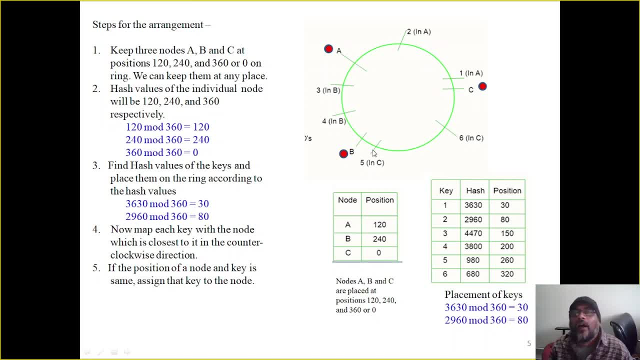 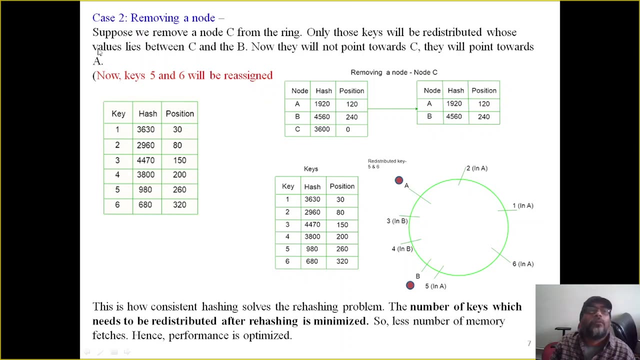 assigned to A. now this is removed. so 5 and 6: these two keys will be assigned to A in place of C now. so you see here, so now they will point to C. so point key 5 and 6 will be reassigned. this key 5 and key 6. 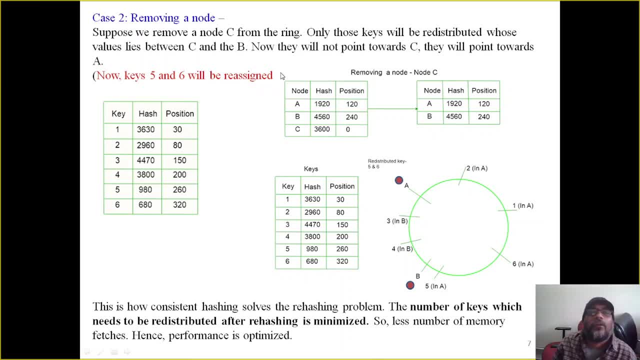 will be reassigned. ok, and they will be assigned now to A. it is written now. they will not point to C, they will point towards A, so rest. other redistribution will not be going to be affected. only this set of key will have to be changed or the key is falling in this range. 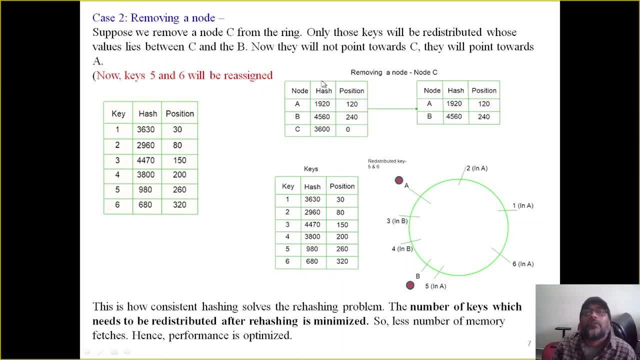 so this is: this is node A, B, C, and we have removed this C. so this is the new position on ring of node and here, actually, I should also show here the node: new node, here it is assigned, ok. so this is how consistent has to be. so let us send. 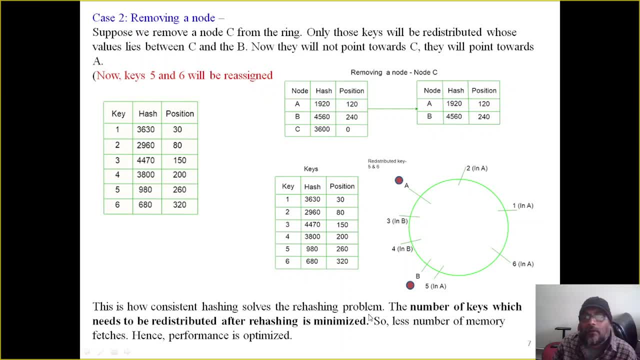 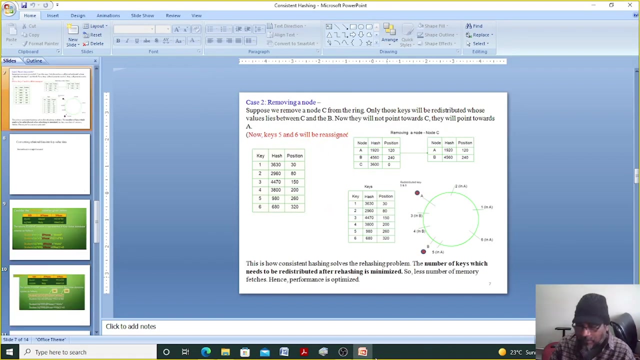 a new key. ok, so this is the new key and this is. this is the new position, which is assumed to be a node C. it can be any. the last we have to. this is the, that is, this is the. this is the the. this is, this is. 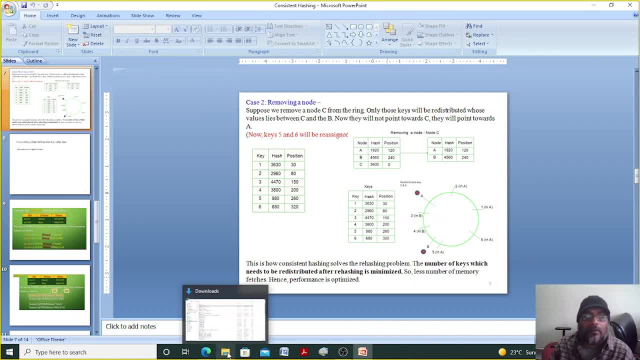 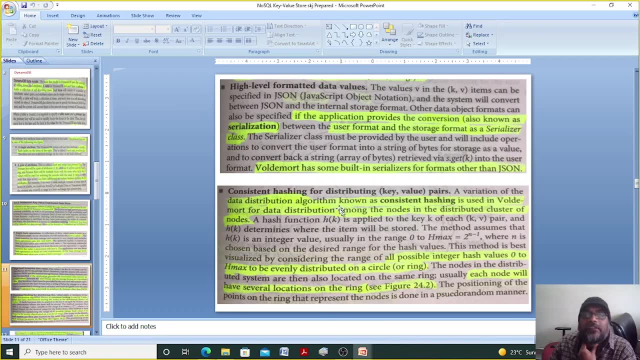 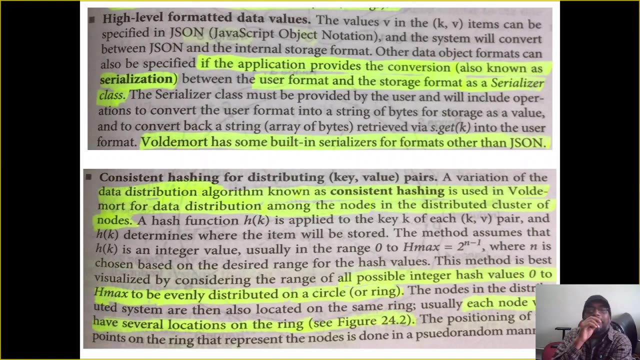 this, this, this. but now we can easily understand that consistent hashing for distributing key value peers, a variation of data distribution algorithm known as consistent hashing, is used for used in Voldemort for data distribution among the nodes in the distributed cluster of nodes we have cluster, the student cluster. we have several notes here and we want two: distribute key value data. 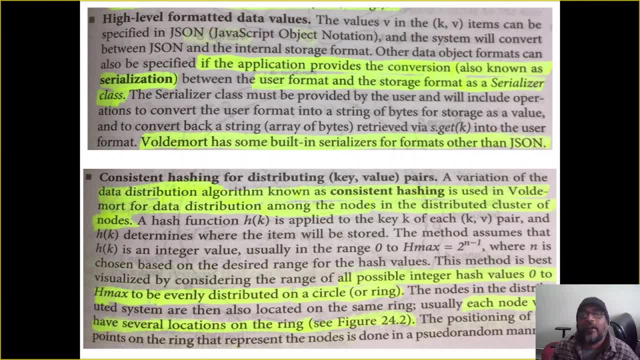 among the ANC. so one algorithm has been designed and this is called consistent hashing. so it is nothing. it is a variation of data distribution algorithm. roughly we can say it is data restoration algorithm. but that distribution algorithm is a legitimate algorithm because it changes a key experimental data 알고 right than for data distribution. игрiden as건 also from data distribution, I read. but 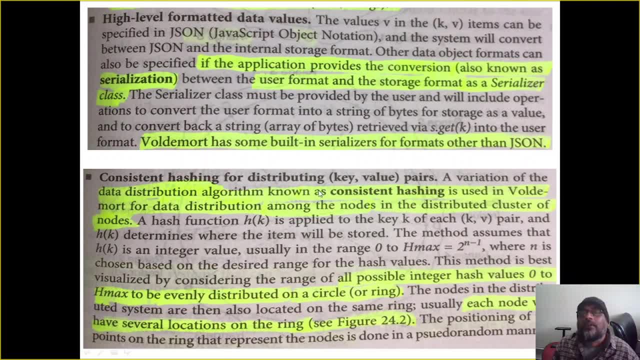 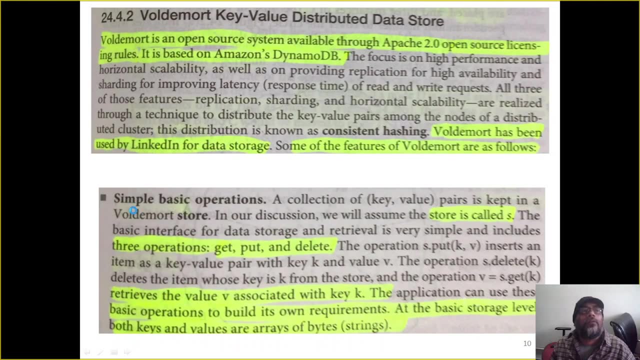 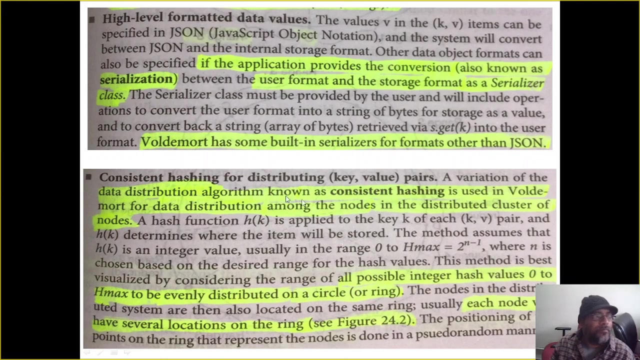 has some feature and ability. so, as consistent hashing is used in Voldemort, this algorithm has been used in this key value database. that was Dynamo DB. this is property of Amazon and this is open source Voldemort. okay, so for understanding that dynamo DB, we do not have details, but this open. 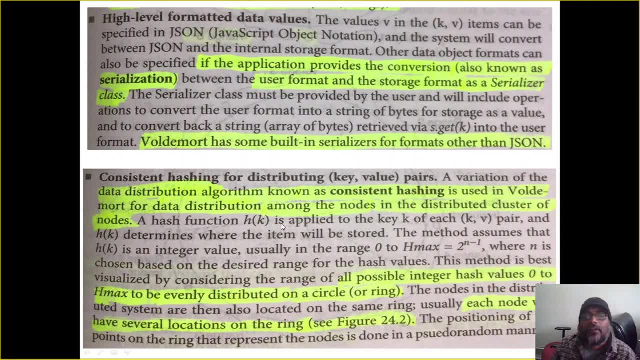 source. it is the same. so a hash function, HK, is applied to the key K of each KD pair. okay, key value pair and sk determines where the item will be stored. hash function: we identify the position where we have to store the map. The method assumes that hk is an integer value, usually in a range of 0 to hmax. some value, that is to be power of 2.. So this is the range where we have to generate the value. The value will be generated by the hash function. 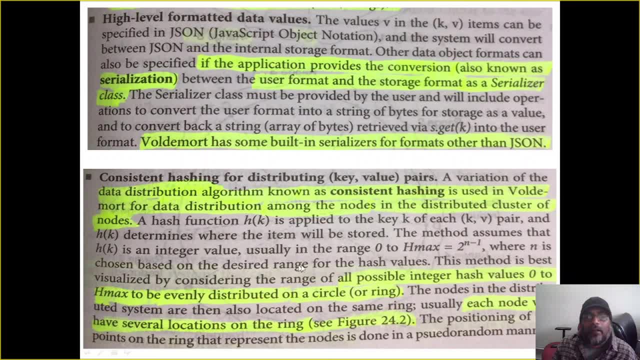 Where n is chosen based on the desired range for the hash values. The method is best visualized by considering the range of all possible integer hash values, 0 to hmax, to be evenly distributed on circle or ring. The nodes in the distributed system are then also located. 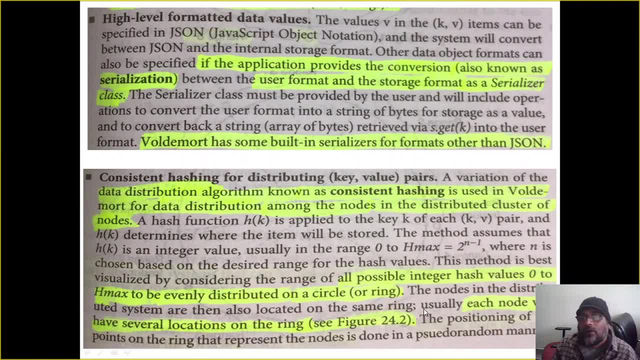 Usually each node will have several locations on the ring. The positioning of the points on the ring that represent the nodes is done in a pseudo-random manner. How do we define random? Random is a natural phenomenon. Nobody can predict it. But if we have to develop some kind of a similar kind of some values that we have randomness in nature but those values are being generated by computer using some algorithm, 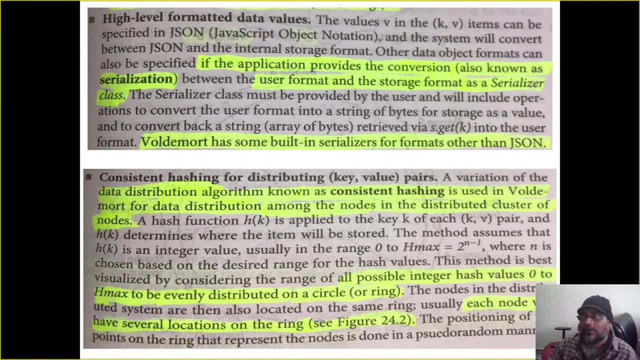 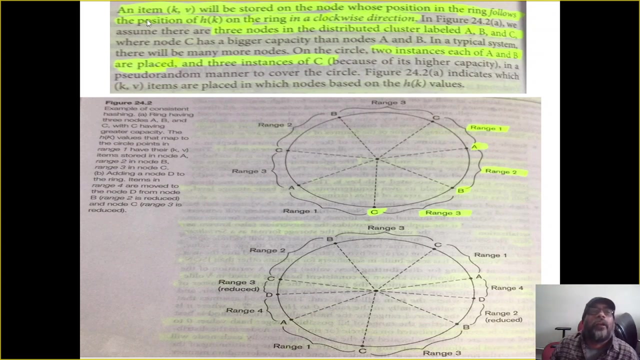 So somebody can argue that it is not true random, it is pseudo-random, So pseudo-random word is used in practice. So the positioning of the points on the ring that represent the nodes is done in a pseudo-random manner. An item kv will be stored on the node whose position in the ring follows the position of hk on the ring in a clockwise direction. 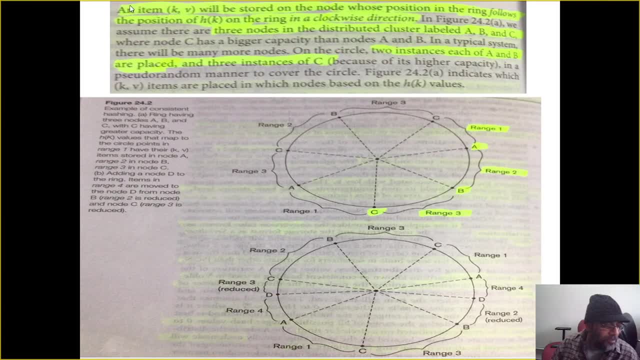 Here clockwise is written, So there is no question, clockwise anticlockwise, So any convention can be used. So in this figure we assume there are three nodes in the distributed cluster labeled abc, where node c has a bigger capacity than node a and b. 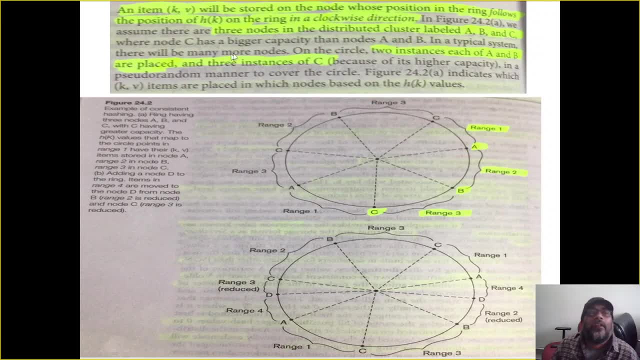 So in a typical system there will be many more nodes on the circle. Two instances of a and b are placed Here. a and b are placed Here. b are two nodes and they are replications or instances. Instances means they are also a node. 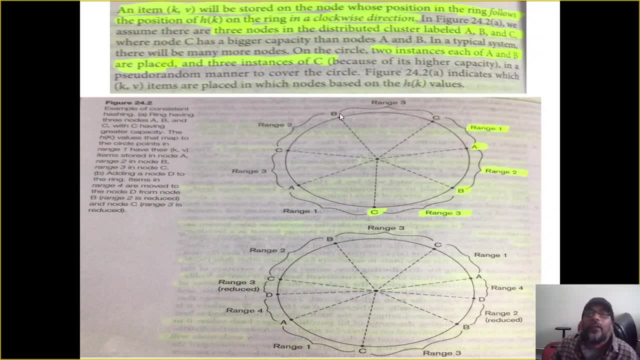 So a and b, they have been copied. Actually copy is not exactly saying copy, It is another node. But for software, For software it is, and for hardware two issues comes here. So logically it is same, but physically it is different. This is correct explanation, logically. 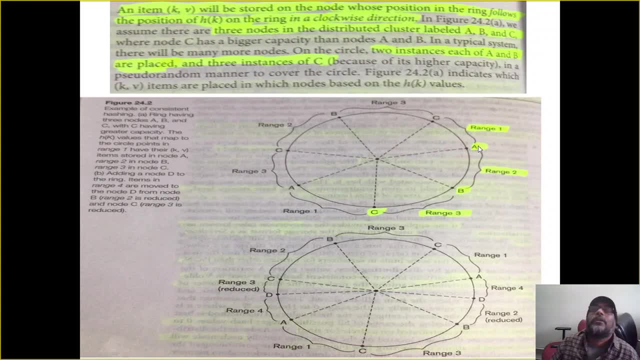 Or it is instance of. somebody can argue it is a node, a node, a type node. Ok, So we assume there are three nodes in the distributed cluster labeled abc. In the distributed cluster labeled abc, where c has a bigger capacity than node a and b. 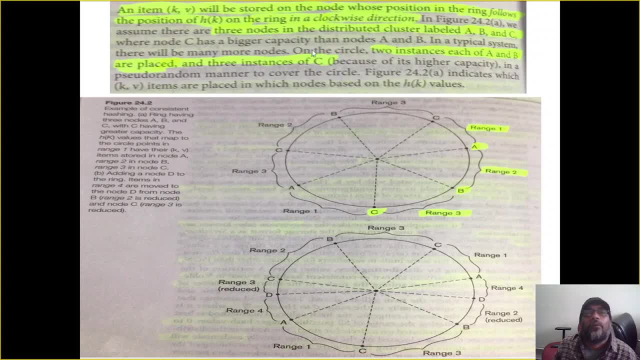 In a typical system there will be many more nodes on the circle. Two instances of each a and b are placed and three instances c because it is higher capacity. So in a pseudo random manner to cover the circle, figure a indicates which kv items are placed. 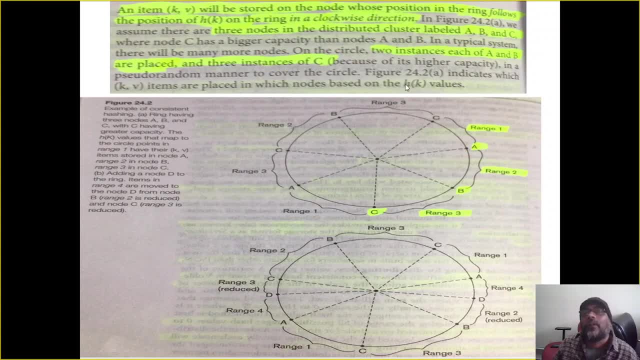 In which node, based on the h key value. You see, here this is abc and here you see, this is c, this is b, this is another c. So three copies of c are here and two copies of b are present here. When we say a node, we correspondingly define the range of values. 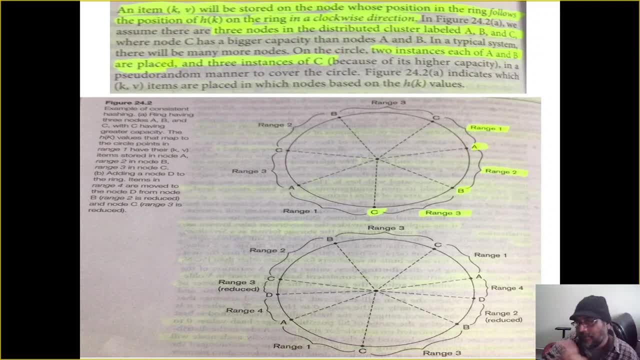 If key is falling in this range, then that will, they will go or they will be stored on this node. So this is shown here. range one to node a. Range two to node b, Range three to node c, like this explanation. So here you see here. similarly for node a, range one is shown here. 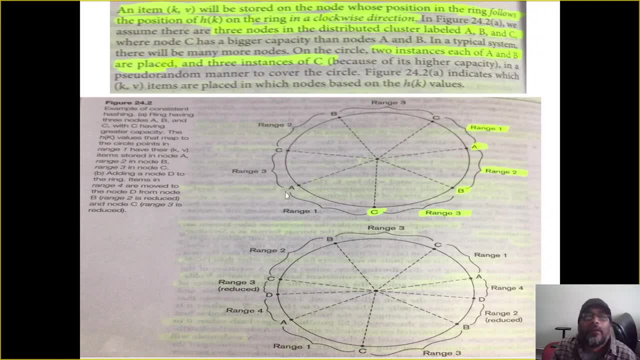 So, similarly, some other place node a is present, then there will be range one. Here it is range one, So if keys are falling, then they will go to this node. Ok, And this is situation when Node is added. So we will discuss this diagram later. 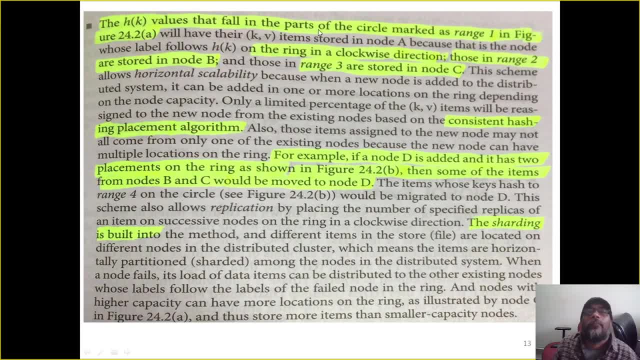 The h key values that fall in the parts of the circle marked as range one in the figure a Will have their key value items stored in the node a. Ok, Because That is the node Whose level follows h, k on the ring in the clockwise direction. 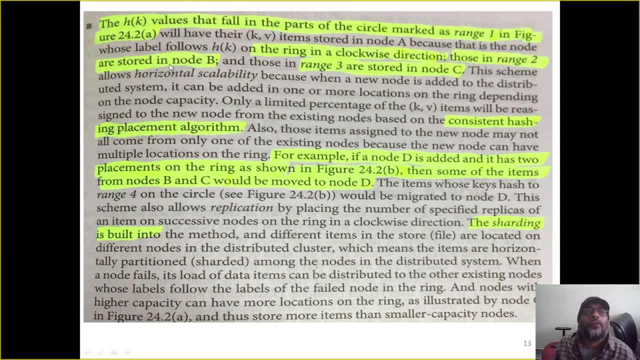 Those in range two are stored in node b And those in range three are stored in node c. Ok So, range one key, range two, key range two keys and range three keys. They are stored at node a, b and c. 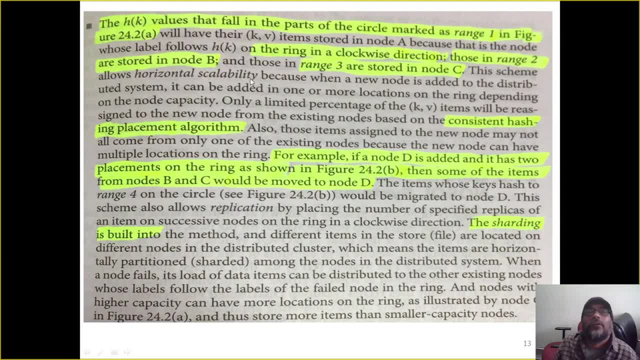 This scheme Also called horizontal scheme, Horizontal scaling, Because when a new node is added to distributed system, It can be added in one or more location on the ring, Depending on the node capacity. Only a limited percentage of kv items will be reassigned. 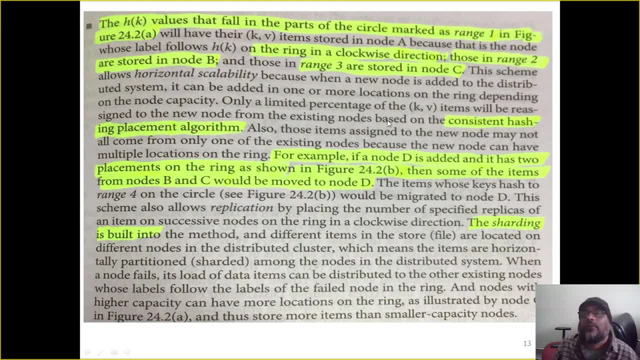 To the new node from the existing node, Based on the consistent hashing placement algorithm. Also, Those items assigned to the new node may not All come from only one of the existing nodes, Because the new node can have multiple locations on the ring. 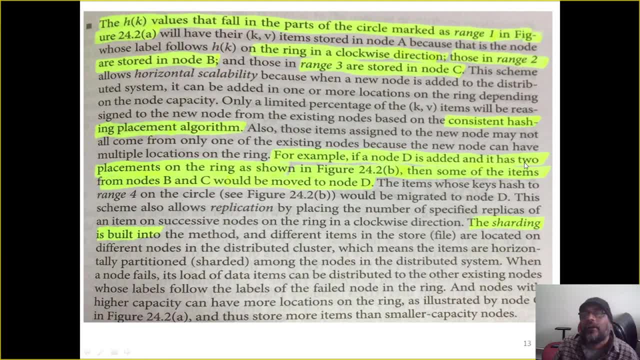 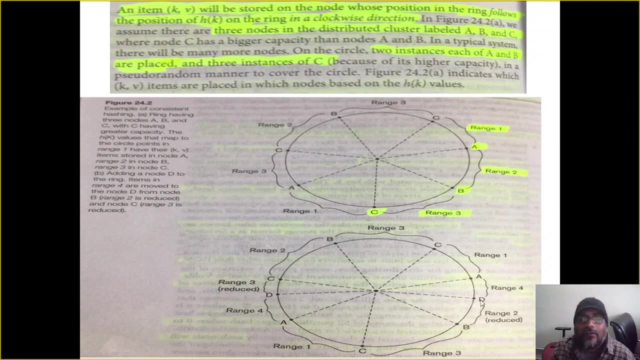 For example, Node d is added And it has two placements on ring, as shown in figure b. Ok, Now d node has been added And it is added at two places. This is d node You see here, And this is another d node. 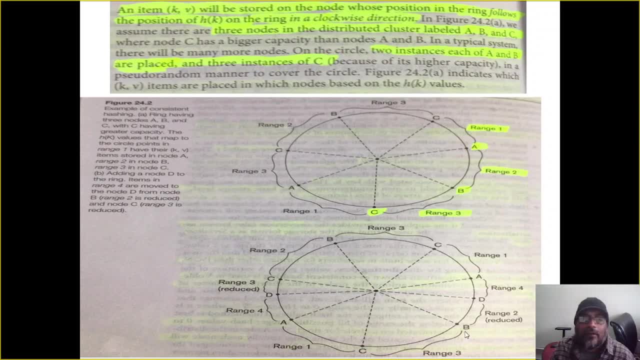 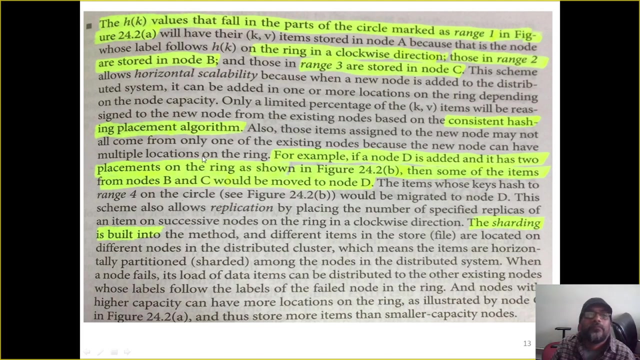 Ok, It is between a and b here. Ok, So this is d node here And b c. So, for example, For example, If d node is added two placements on the ring, As shown in figure b, Then some of the items from node b and c would be moved to d. 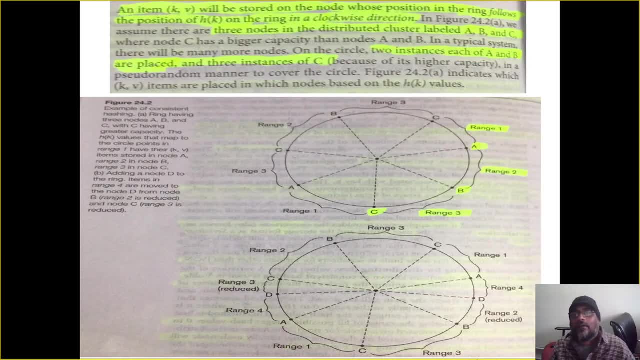 So what will happen when we add here Then few items of which is saying b? So you see here, If we make rule then to go clockwise direction and anticlockwise. So one explanation here is wrong In this book. So you see here: 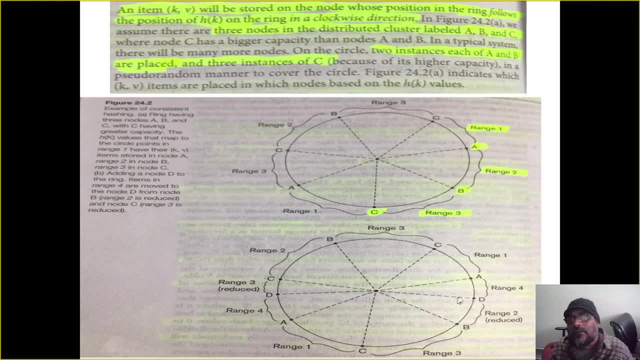 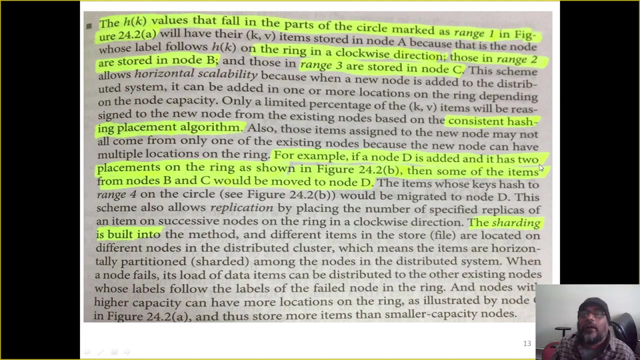 If we make rule of clockwise direction, Then what will happen? A key data of a will be This d. This d is added here. So Just a minute First I read, Then I will come here. D is added And it has two placements on the ring. 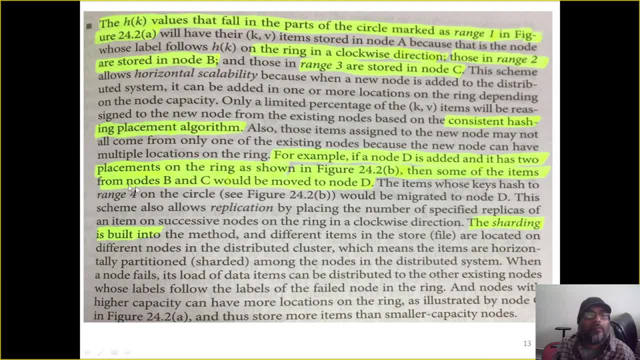 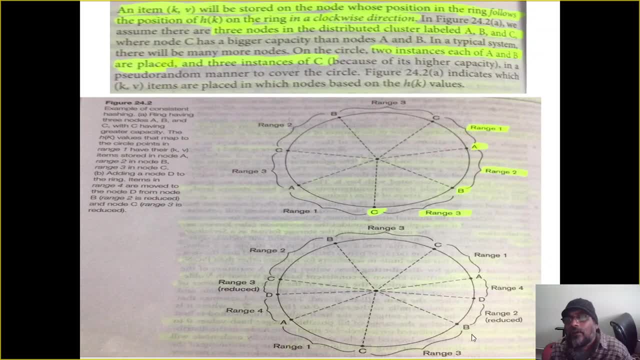 As shown This, then some of the items from node b and c would be moved to d From b and c. it is saying So. So d is here And d is here. So it is saying some data from b will be moved here. 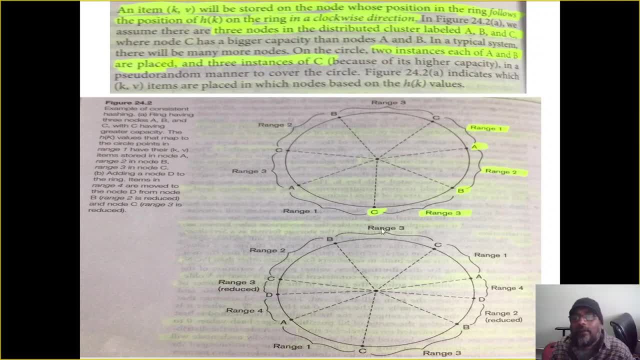 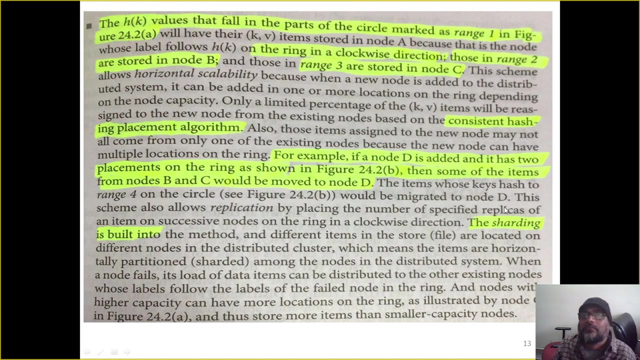 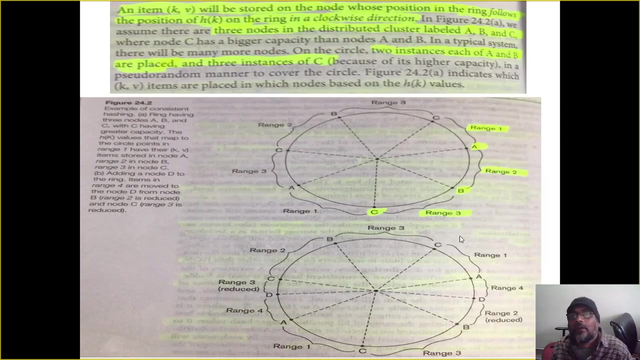 So if we make rule Then we go To clockwise So as per the convention of clockwise Data Data of Equal, The item whose key has Range four on circle c Would be migrated To node d, Range four. 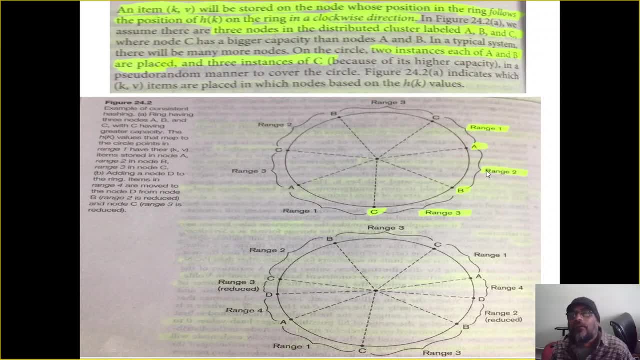 Range one, Range one, Range two. Now This range. When we add d, Then it is the range four. Okay, And this range b is this one. So Some data From B To d Will be moved. 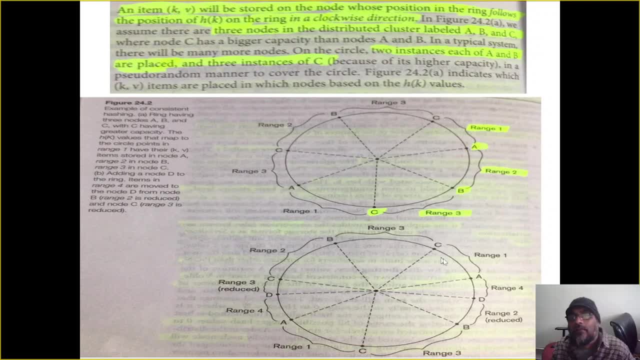 So When we say This, When we move this one, Actually there is a mistake: clockwise and anticlockwise, So The explanation comes Using clockwise Here, So it It is also written Somewhere. I am coming here. 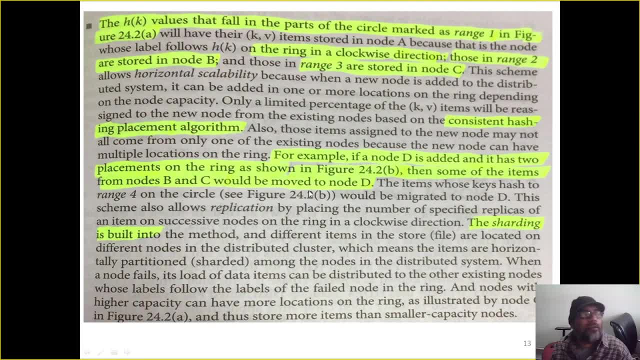 So there is no confusion. Clarity is there, But only Some Convention issue, So there is no problem. So don't be confused here. The item whose keys has Range four On the circle Would be migrated To d. 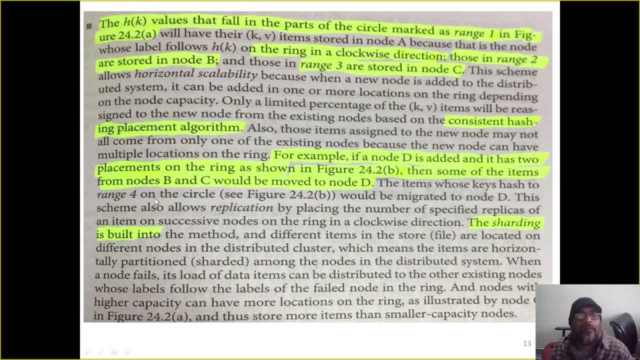 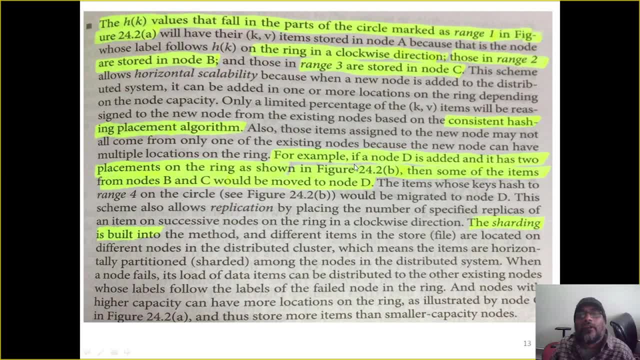 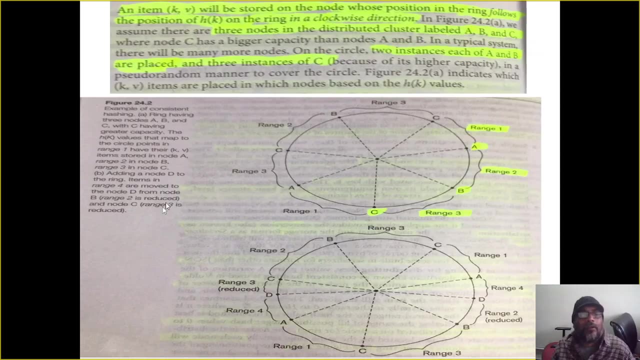 The item Of An Item, Some Thing I Started From Here. For Example, If nodes Is Added And so these item range C is reduced and it is written here: C, this will move the item will. 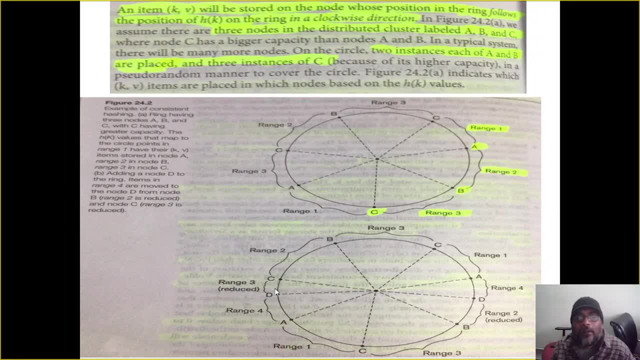 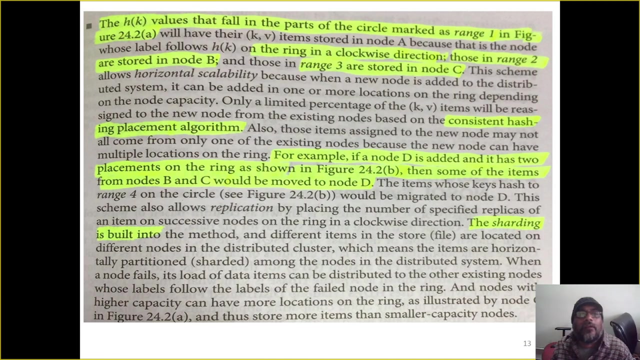 be moved only when: if we move in anticlockwise ok. similarly, here this B item will be moved to D. if we make rule of anticlockwise ok data which is close to the node, when we move anticlockwise, then B, this C data will be moved to C, to D, B and C. from B and C. 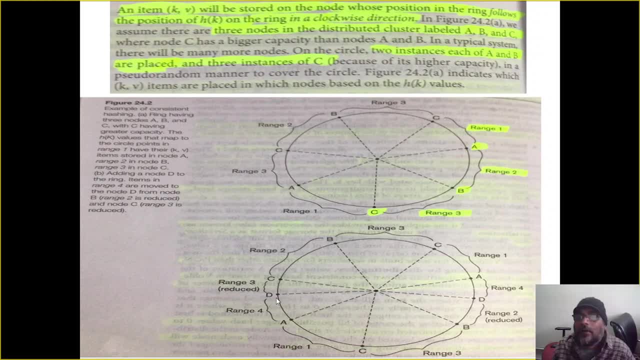 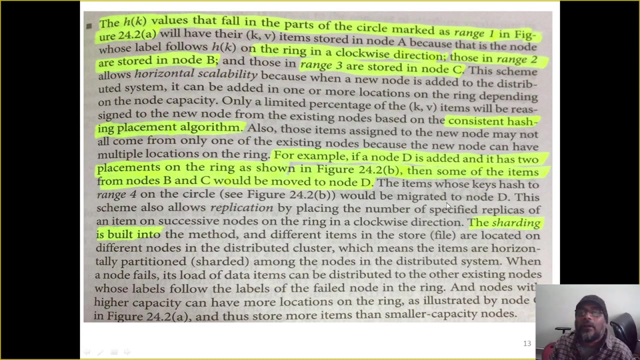 So from C here and from B here. ok, it will be only when we have anticlockwise. ok, but here they have taken clockwise. so that is some, I think, mistake may be, but understanding issue, there is no problem. Migrated to node D. This scheme also allows that. 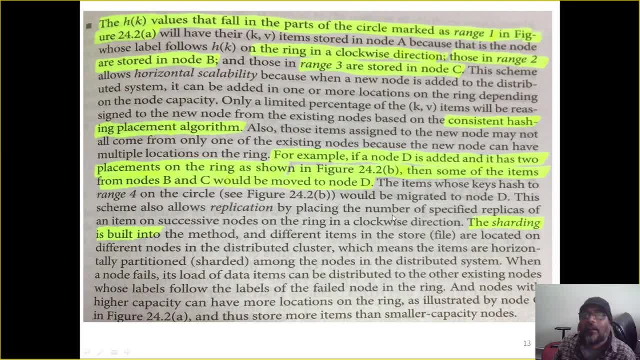 So we can do replication by placing the number of specified replicas of an item on successive nodes on the ring in clockwise direction. ok, so the sharding is built. sharding means dividing data on several nodes. so how sharding is done. so this is technique: the sharding is built. 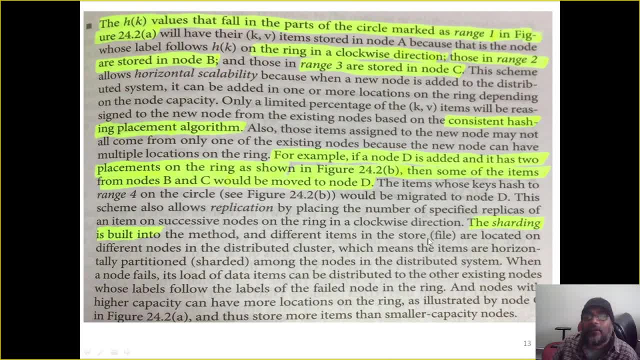 into the method And different items in the stored file are located on different nodes in the distributed cluster, which means the items are horizontally partitioned or sharded or distributed among the nodes in the distributed system. in this way we have very large volume of data and 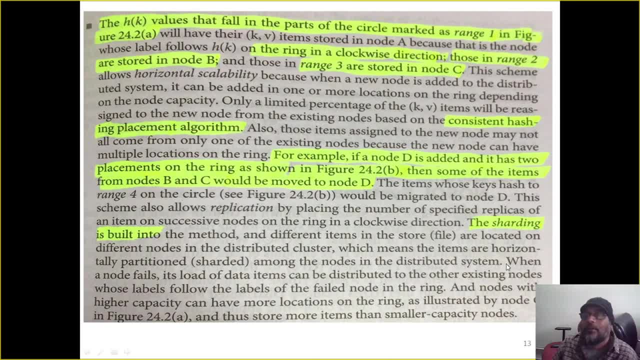 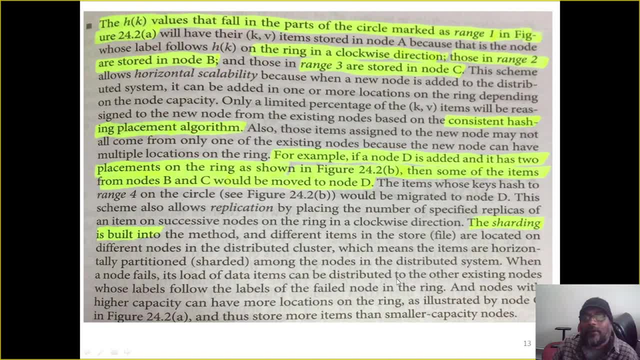 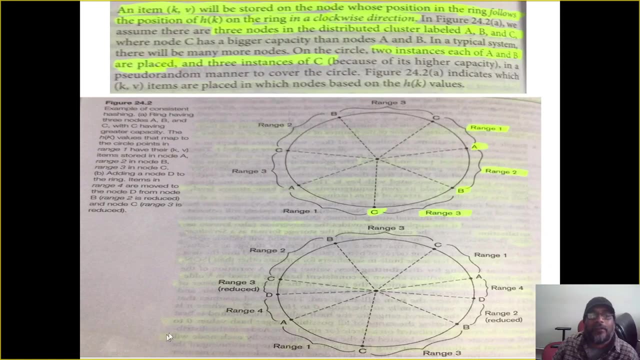 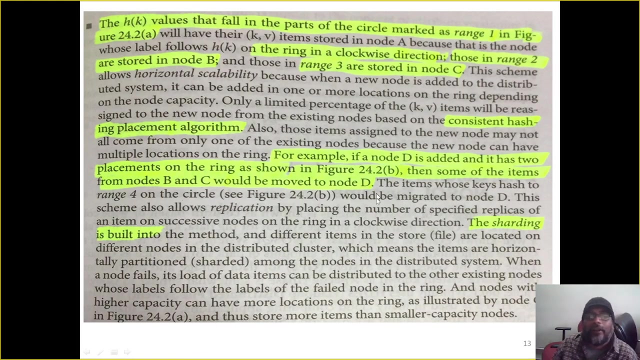 When a node is distributed. When a node is distributed, Then the then the same named data, named load can be used. So In the ring end nodes, which with higher capacity, can have more locations on the ring, as illustrated by C, thus store items than the smaller capacity nodes. 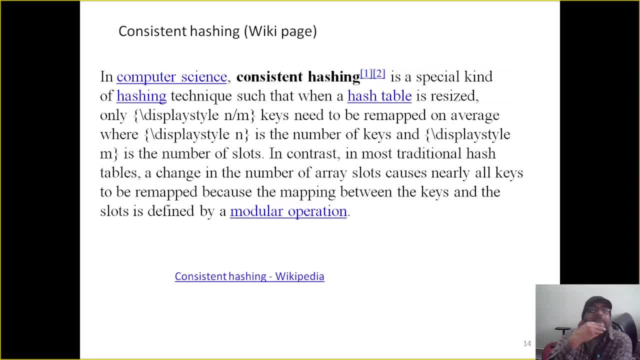 Consistent hashing is a special kind of hashing technique such that when hash table is resized Here when we add or remove node. so basically hash size is going to be changed, But in consistent hashing when node is added or removed, The reassigning remains the same, Remains unaffected, or if it is going to be affected, then only a limited number of items have to be reassigned. 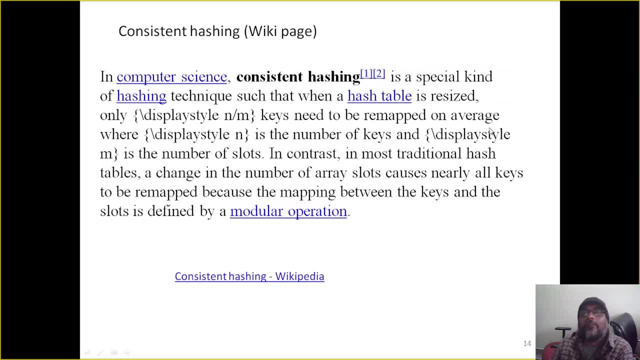 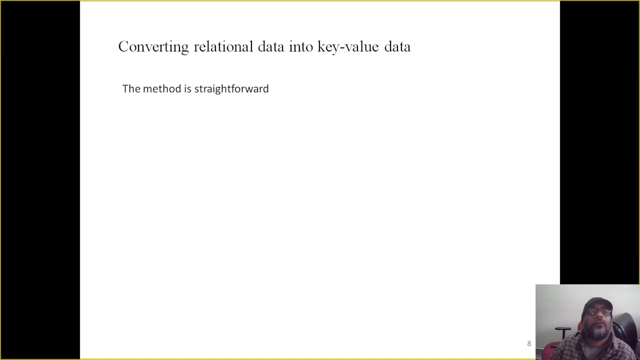 Resized. only Key need to be remapped on average. where is the number of keys and the number of slots? In contrast, most traditional hash tables are changed in the number of arrays. slot causes nearly all keys to be remapped. Now we come. This is very simple: how relational data can be converted into key value data. 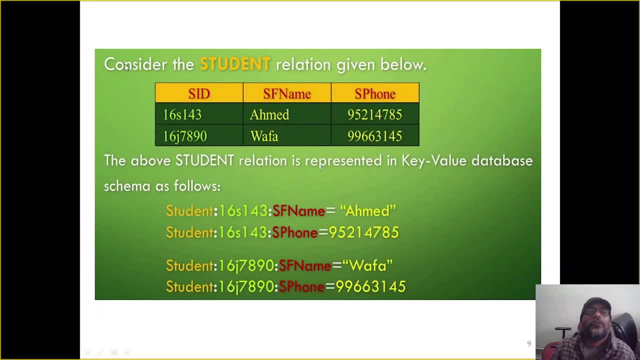 So method is straight forward. Suppose this is one student relation or table And it has two triples: student id key, student first name and student phone number. The student relation is represented key value database. like Student, this is the this key value And first name. Okay, second, this key value and this phone number.